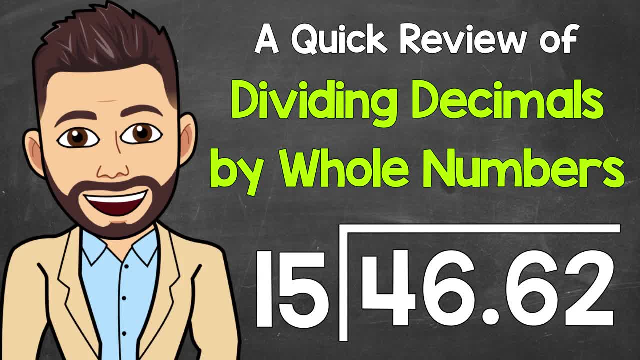 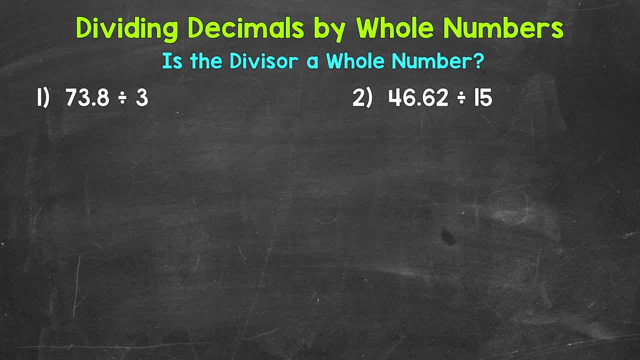 Welcome to Math with Mr J. In this video, I'm going to cover how to divide decimals by whole numbers. Now, decimals and division show up all throughout math and really throughout life as well. So being able to work with decimals and solve division problems involving decimals, 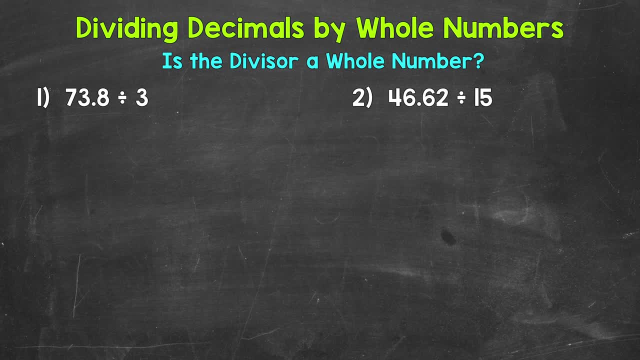 will be beneficial, no matter what class level of math or goal you are working towards. Whatever your situation may be, this should be helpful in better understanding how to divide decimals. Let's jump into number one, where we have 73 and 8 tenths divided by 3.. 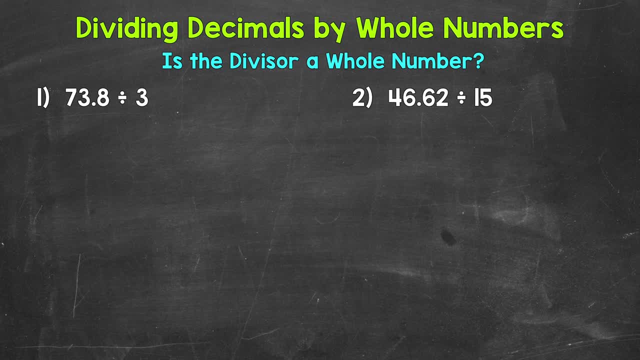 The first thing that we need to do is set this problem up. That way we can go through the division process. 73 and 8 tenths is the dividend, the number we are dividing, So it goes under the division bar 73 and 8 tenths divided by 3.. 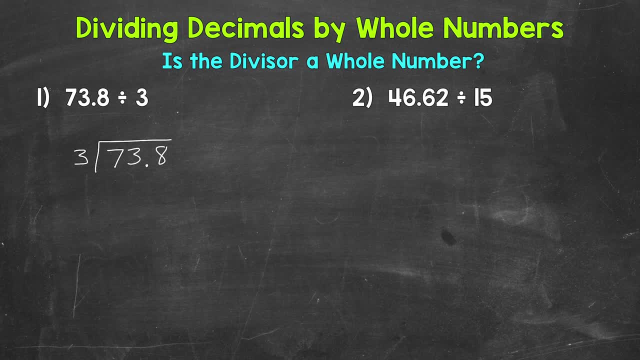 3 is the divisor the number we are dividing by. It goes on the outside of the division bar. Now, whenever we have a division problem that involves decimals, we always need to check: is the divisor a whole number? If yes, bring the decimal straight up into the answer. 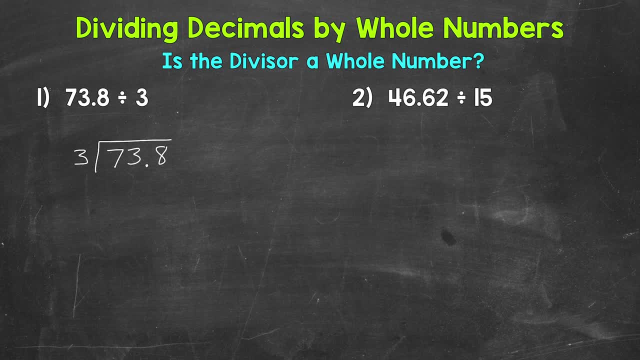 So for number one, our divisor is 3.. That's a whole number. So we bring the decimal straight up into the answer. Now we go through the division process, The same process we use when we divide whole numbers. So divide, multiply, subtract, bring down, repeat. 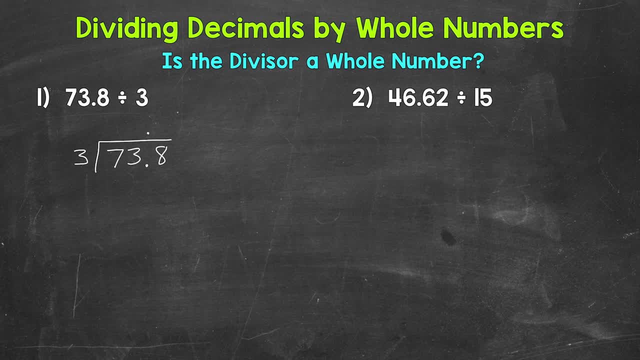 We start with divide. So we have 7 divided by 3. How many whole groups of 3 in 7? Well, 2.. That gets us to 6.. Now we multiply 2 times 3. Is 6.. 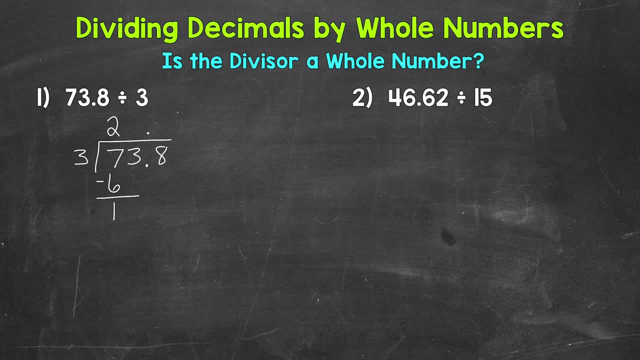 Subtract 7 minus 6 is 1.. And then we bring down: Now we have 13. And we repeat. So we go back to divide 13 divided by 3.. How many whole groups of 3 in 13?? 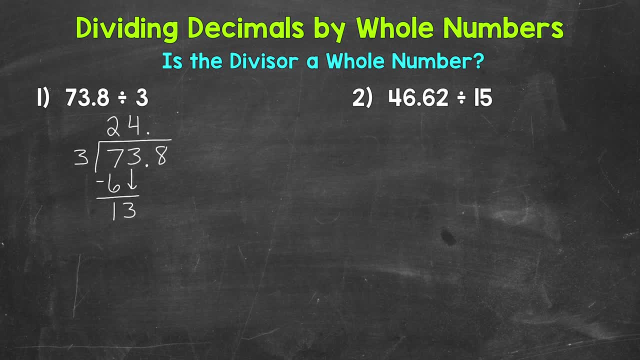 4.. That gets us to 12.. Now we multiply 4 times 3 equals 12.. Subtract 13 minus 12. Is 1.. And then we bring down the 8. Now we have 18. And we repeat. 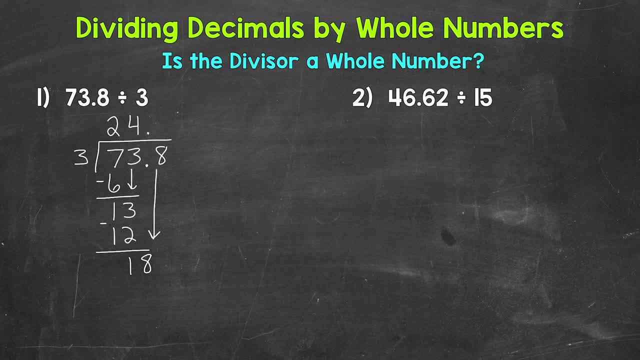 So we go back to divide 18 divided by 3. So how many whole groups of 3 in 18? 6. That equals 18 exactly Multiply 6 times 3.. 18.. Subtract And we get 0.. 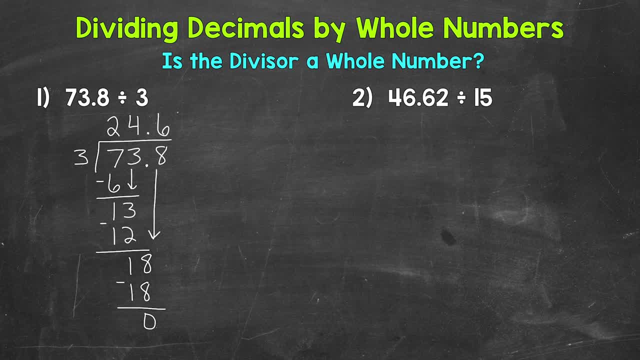 So we went all the way over to the furthest place, Furthest place to the right, which was the tenths place for number 1.. And we have a clean-cut zero here that tells us that we are done. Our final answer: 24 and 6 tenths. 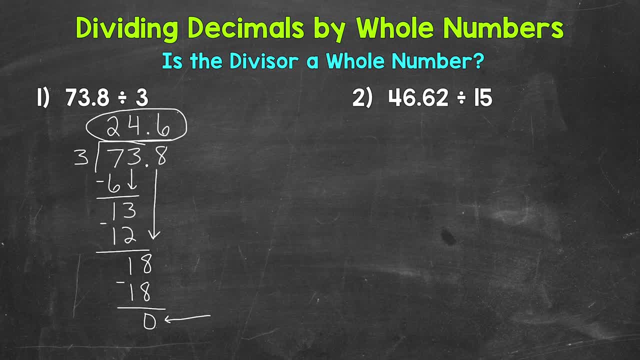 For number 2, we will see what happens when we do not get that clean-cut zero and we need to extend the problem until we do. Let's move on to number 2, where we have 46 and 62 hundredths divided by 15.. 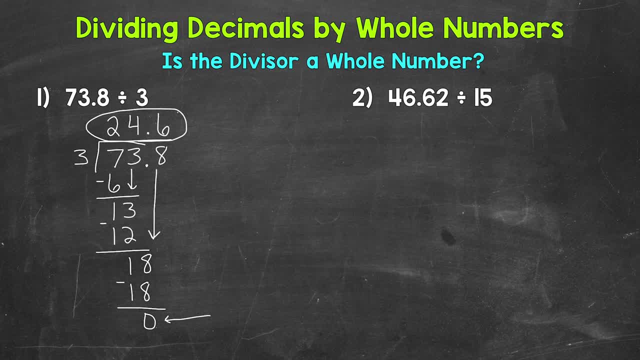 Let's move on to number 2, where we have 46 and 62 hundredths divided by 15.. Let's move on to number 2, where we have 46 and 62 hundredths divided by 15.. Let's start by setting this problem up. 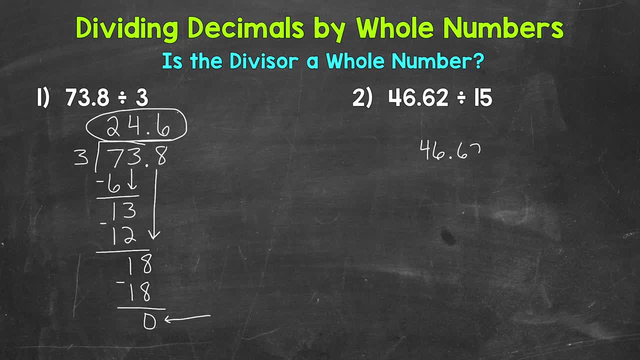 46 and 62 hundredths divided by 15.. Is the divisor a whole number? Yes, 15 is a whole number. That means we bring the decimal straight up into the answer And now we go through the division process. So we start with divide. 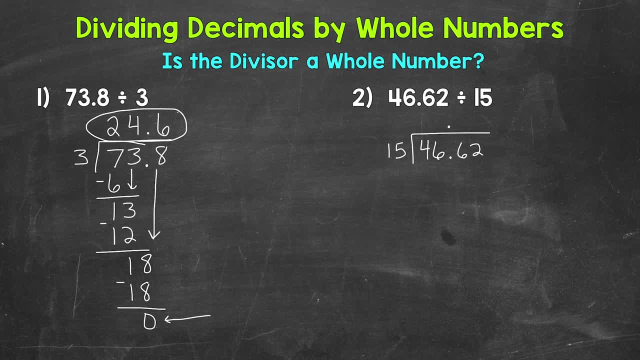 We have 4 divided by 15. How many whole groups of 15 in 15?? Well, we can't do that, So we need to use the 6 as well and take a look at 46. We have 46 divided by 15.. 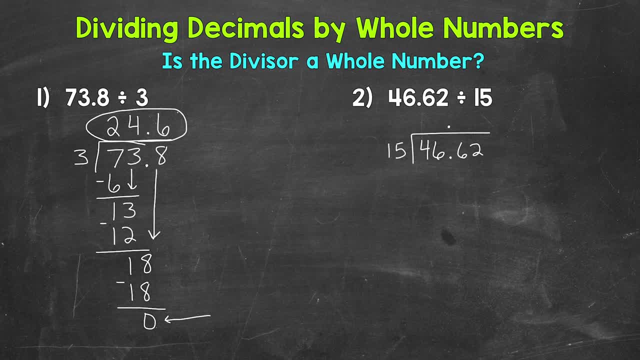 How many whole groups of 15 in 46?? Well, 3. That gets us to 45.. Make sure that 3 goes above the 6 in 46, not above the 4. Since we used both of those digits and we had 46 divided by 15, that 3 needs to go above. 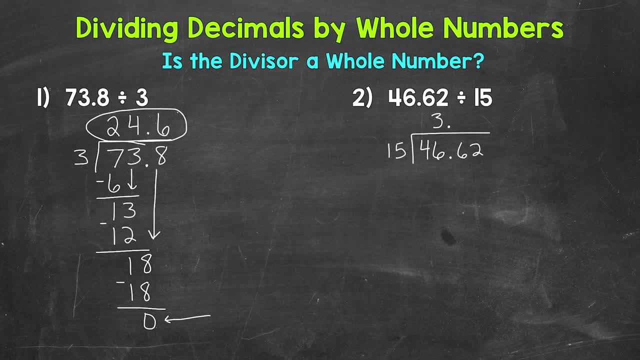 the 6.. Now we multiply 3 times 15 is 45.. Subtract 46 minus 45 is 1.. And then bring down: Now we have 16, and we repeat. So back to divide: 16 divided by 15.. 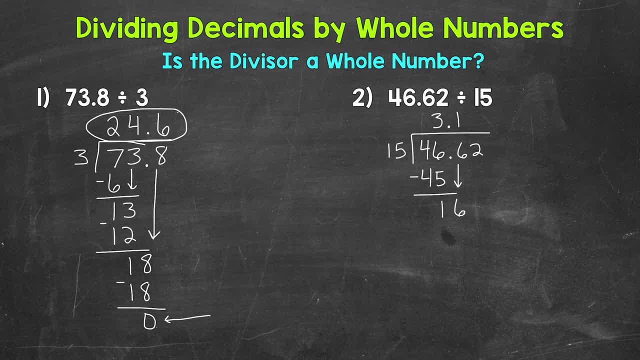 How many whole groups of 15 in 16? 1. Now we multiply 1 times 15 is 15.. Subtract 1.. Subtract 16 minus 15 is 1.. Bring down the 2. And now we have 12.. 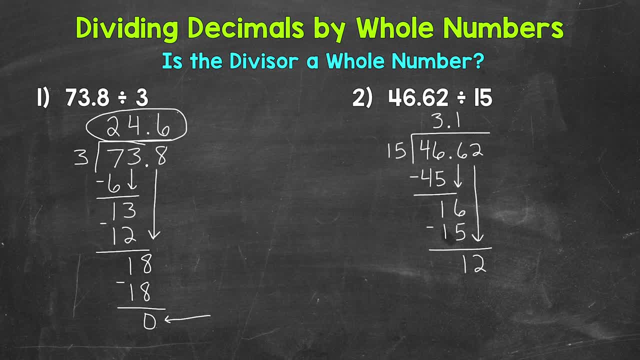 So repeat And we go back to divide: 12 divided by 15.. How many whole groups of 15 in 12?? Well, we can't do that, So we need a 0 here And now. we multiply 0 times 15 is 0.. 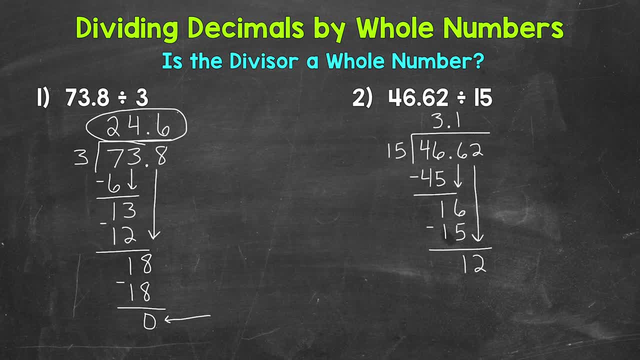 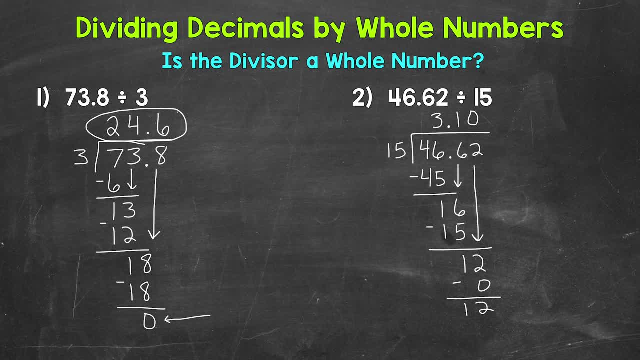 Subtract Construct: 저�행 가여 12 돼야 �表 이�usion 1.. So we went all the way over to the furthest place, to the right, the hundredths place, But we have a 12 at the end. 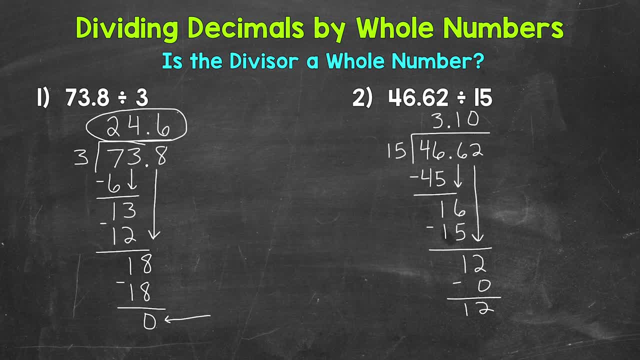 We do not have a clean cut 0 yet. That 12 does not mean remainder 12 – like when we work with whole numbers. This answer is in decimal form, so we need to keep it that way. What we need to do is extend the problem until we do get a clean cut 0, and that will mean 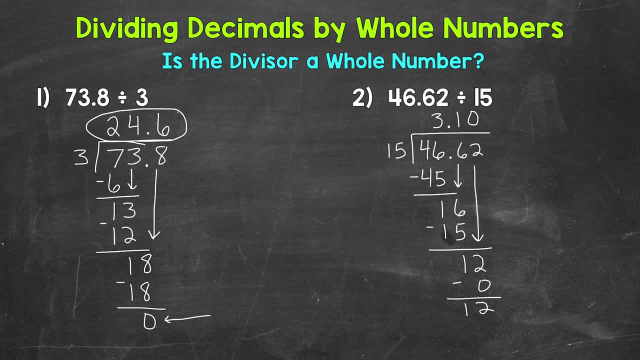 The problem is done and we have our final answer. We can do this by using placeholder zeros that we can bring down. So let's use a placeholder zero in the thousandths place that we can bring down and continue this problem in order to work towards that final answer. 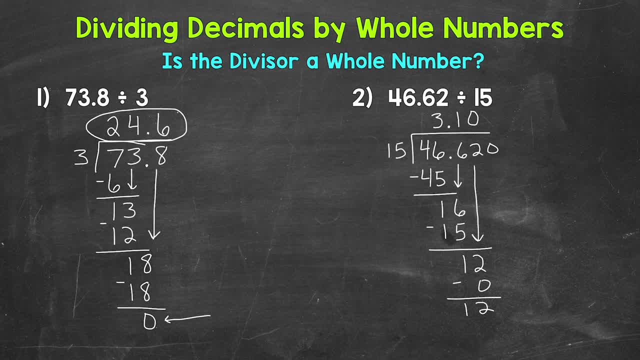 Now remember, zeros to the right of a decimal do not change the value of that decimal, of that number. So we are able to use this strategy. Let's bring this zero down and continue the problem. So now we have 120 and we repeat.